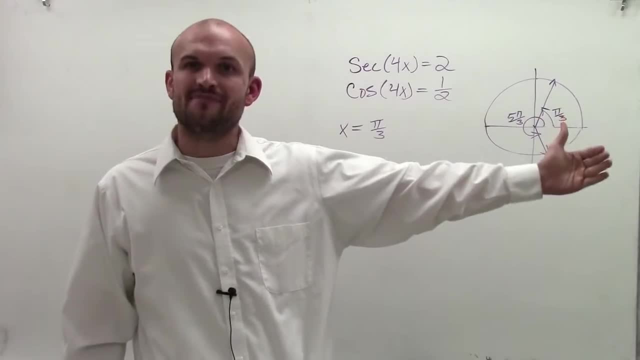 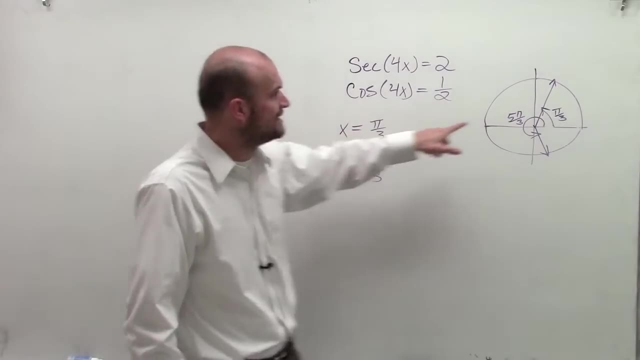 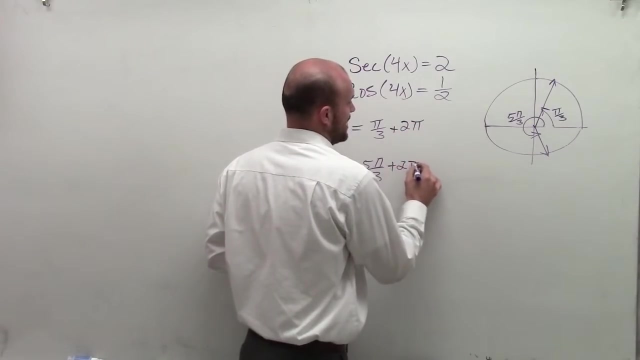 because, remember, the cosine and secant graph continue infinitely in the positive-negative direction. So therefore, to find the values of x equals 5, pi over 3 and pi over 3, I need to keep on adding coterminal angles. So therefore I'm going to add 2 pi plus 2 pi. 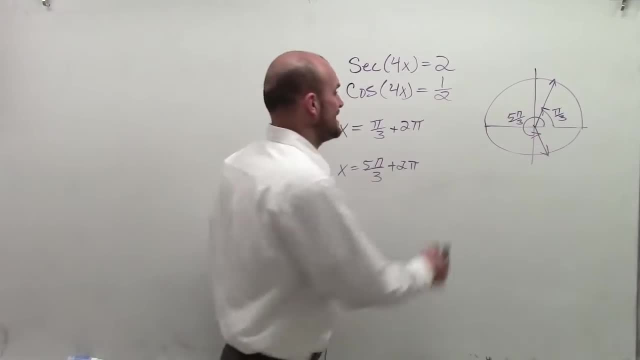 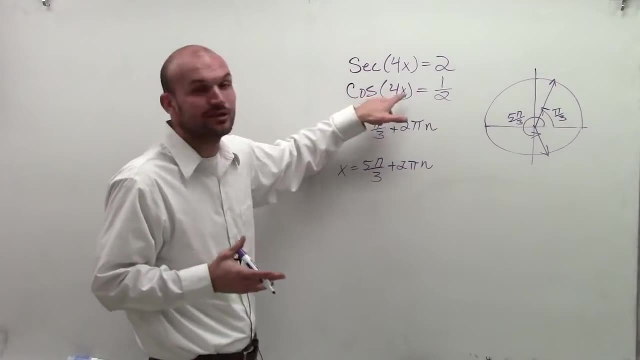 And I can keep on doing that in the positive-negative direction infinitely times. So we're going to use a variable to represent that. So we're going to use a variable to represent the infinite many times. However, we're not just solving for x. 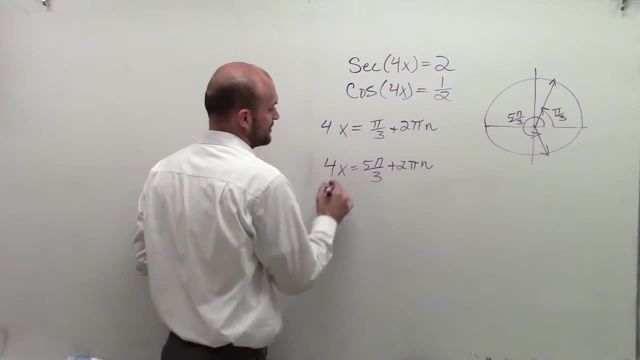 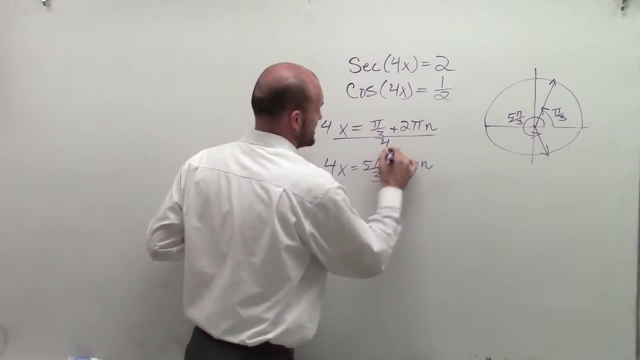 because we look at this, going back to your function, It says when f of x equals 4x. So really my equations are saying 4x equals pi over 3 plus 2 pi n. So therefore I now need to solve for x. 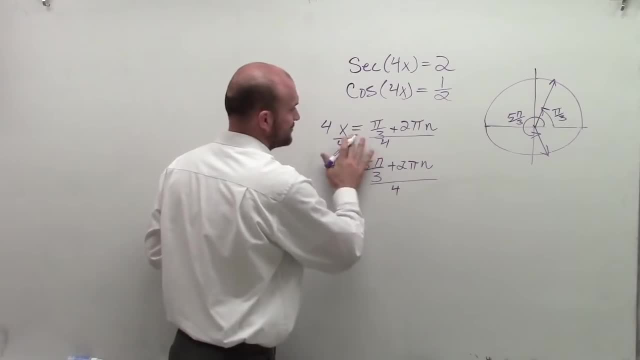 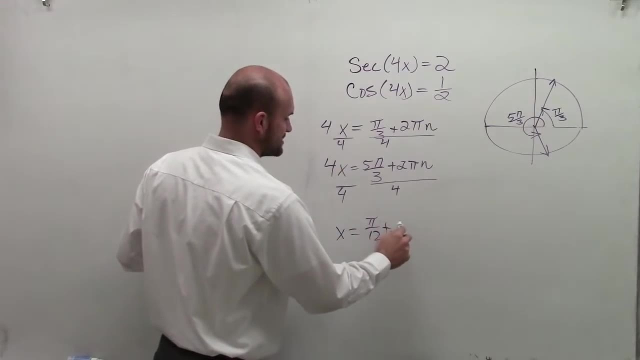 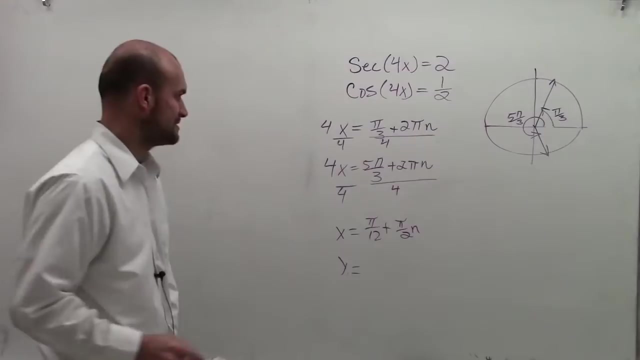 by dividing by 4 on both sides. I don't know why I did my division sign all the way over And therefore I get x equals pi over 12, pi halves n. and then I get x equals and let's see that's going to be 5 pi over 12, plus pi halves n. 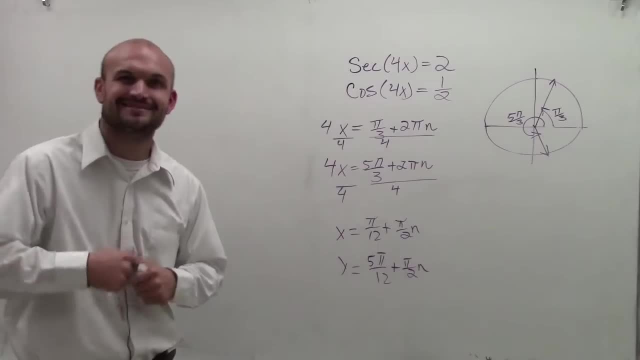 So there you go, ladies and gentlemen. That's how you solve for a multiple angle, All right. 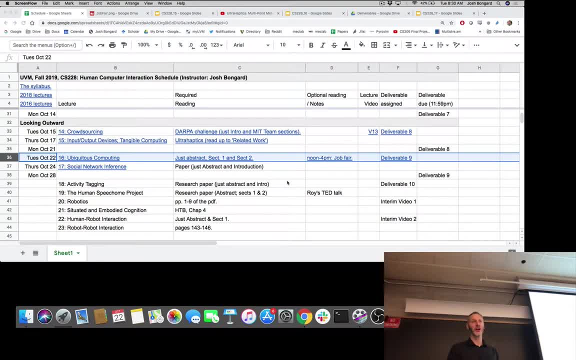 Okay, good morning everybody. Let's get started. I hope you enjoyed Dan Nardi's Q&A session last week. Who wants to go in on a startup? I'm inspired. I don't know about you. All right, great. So let's make sure we understand a little bit about HCI before we start our startup. Back to lecture. We're going to talk about deliverable nine in a moment. We are approaching the end of the deliverables. We are working our way through this theme on 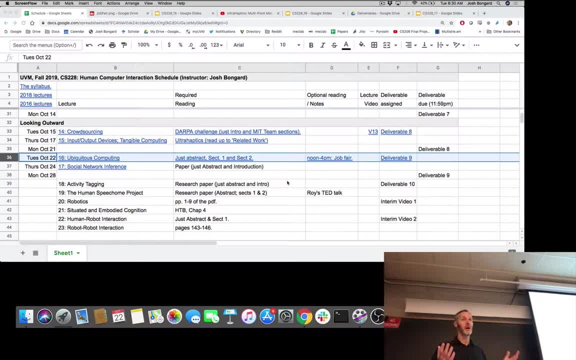 looking outward, So thinking about not just creating pretty websites, but thinking about designing technology which is interacting in real time, in the real world, alongside their human users, And we're looking at some of the unique challenges and opportunities that such ubiquitous computing affords. Just a reminder: today, noon to 4 pm- I'm sure you've heard this-